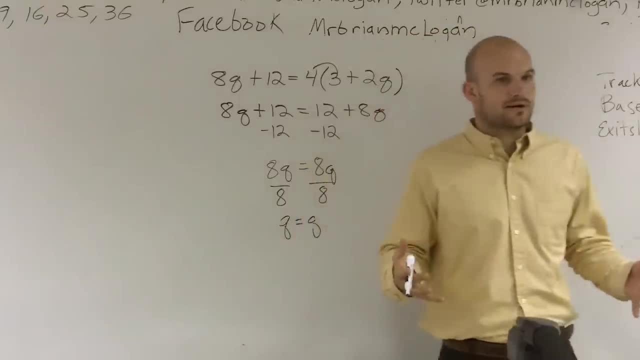 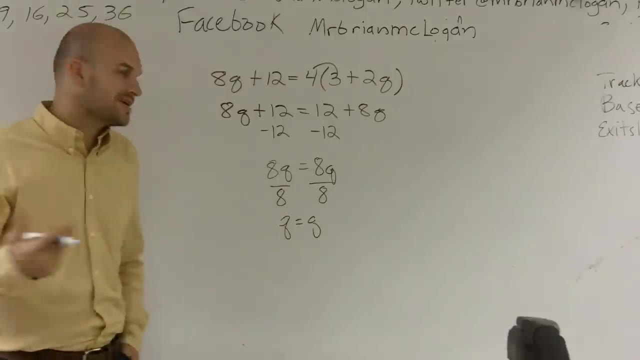 So therefore, my variable doesn't equal exactly one number. And then I say, well, I'm used to like x equals 5, or x equals negative 2. Now I have a variable equals a variable. So what does that mean? 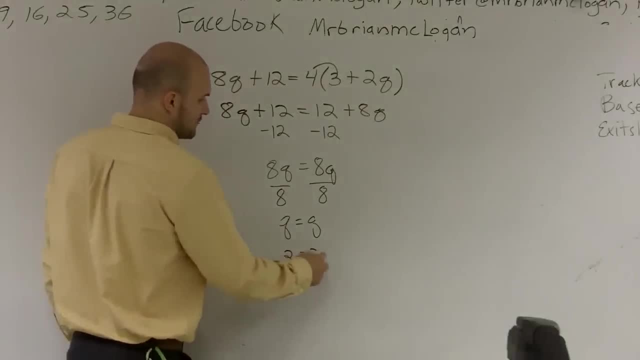 Well, let's pretend q equals 3.. Then 3 would equal 3.. And is that true? Yeah, of course it's always true. What about if I did? 4 is equal to 4? Negative 5 is equal to negative 5.. Therefore, it doesn't matter what value I put in for my variable, It's always going to be true. Therefore, this equation has infinitely many solutions. So there's not just one solution that makes this equation true that we're used to solving, for There's infinitely many. It does not matter what number I put in for x or q in this matter, My equation will always be true. 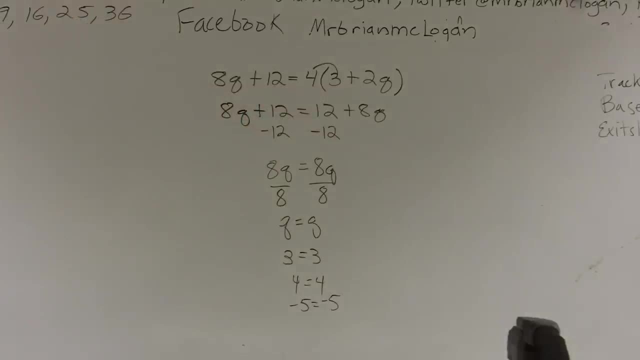 What about if I did? 4 is equal to negative 5?? Negative 5 is equal to negative 5.. Therefore, this equation has infinitely many solutions, So there's not just one solution that makes this equation true. 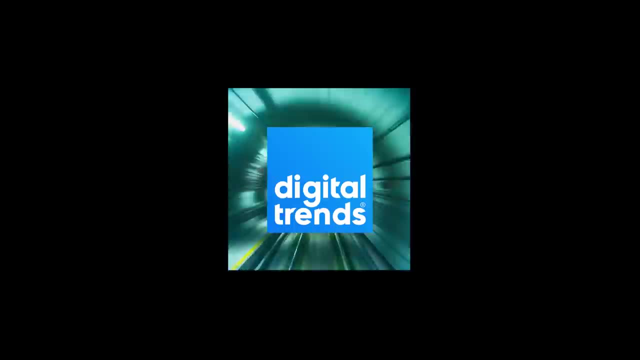 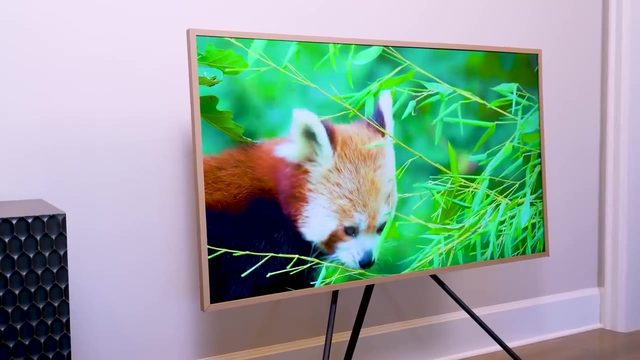 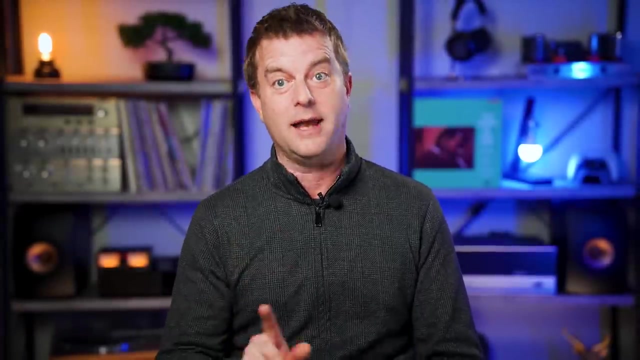 Thanks to Yoshino for sponsoring a portion of our video. What a year it's been for TV reviews. I think we're up to 14 models that we've evaluated and it's no small delight that most of them have been really good, But some are definitely better. 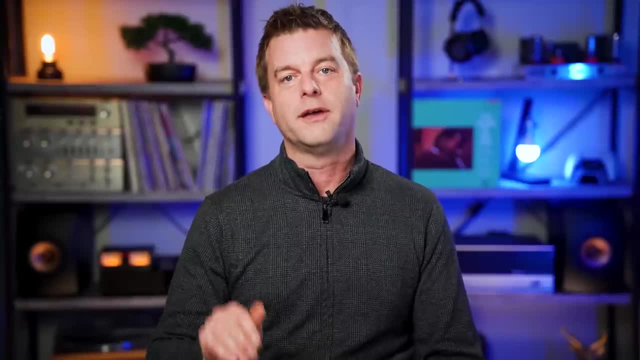 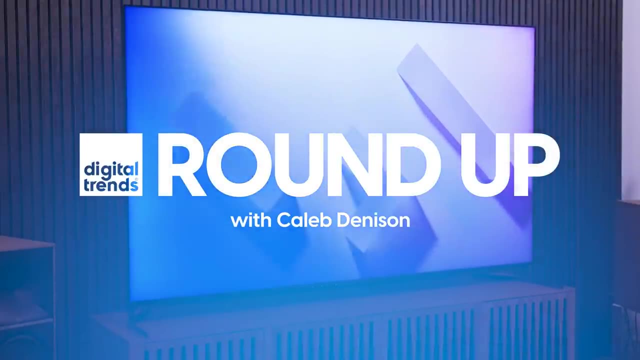 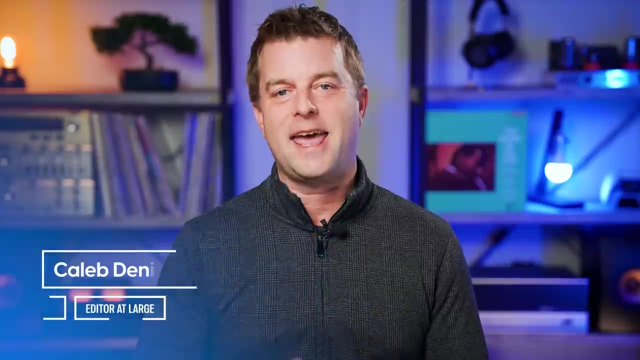 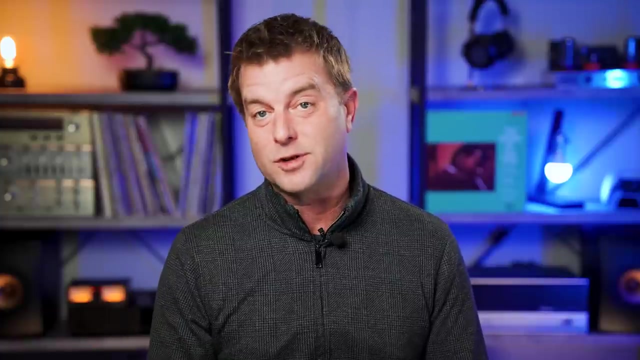 than others and a select few are worthy of being called the best. So let's talk about the best TVs 2023 edition. Welcome back everyone. I'm Caleb Dennison, and whether you're just starting to shop for a new TV and want to build a shortlist, or you're just curious about the best TVs of 2023,, 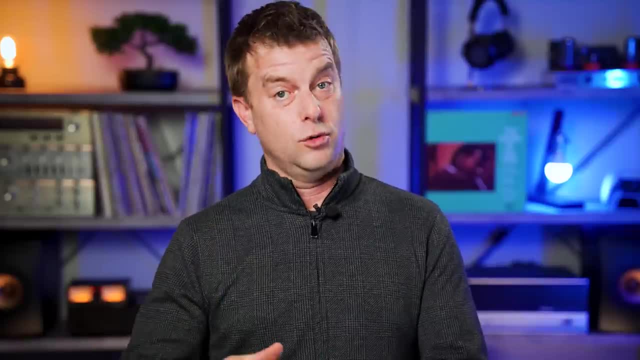 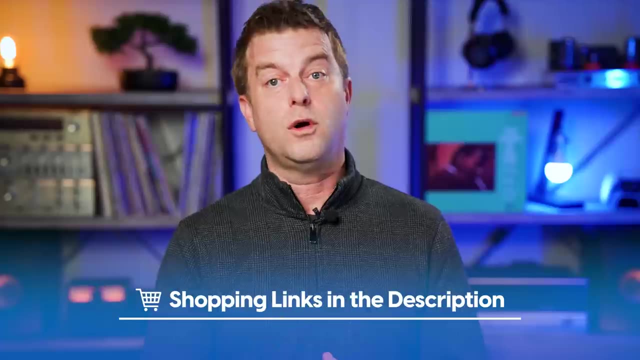 you have landed in the right place. I know many of you who follow this channel may have your ideas around what the best TVs are this year, so let's see if we match up. And for those of you who are just starting to look for a new TV, I'm Caleb Dennison and I'll see you in the next video. 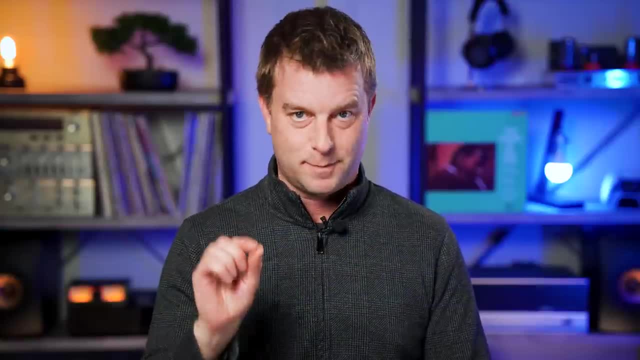 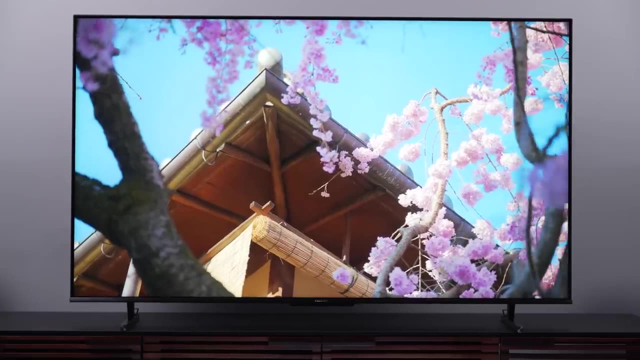 for a new TV and want to build a shortlist, this video is especially for you. My goal is to point you at some specific models and from there you can dive deeper into any of these TVs by checking out our full review for those models, and we'll link to those reviews down in the description to